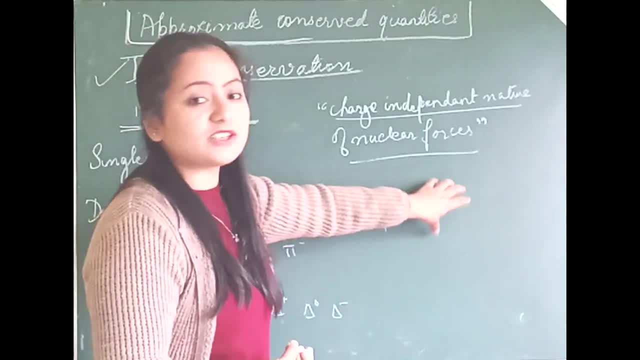 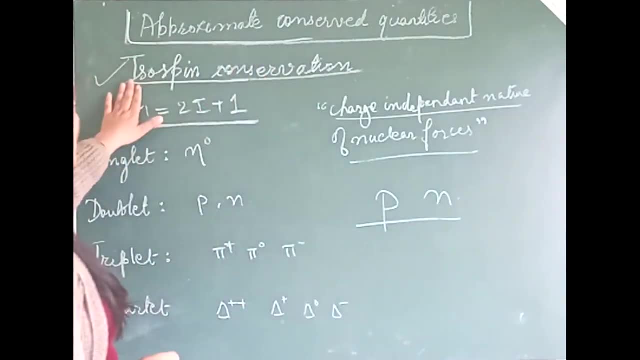 say they cannot identify whether these are charged particles or not. For them both proton and neutron is going to be same. So to avoid that, we introduce the concept of isospin. So isospin is an isospin. Your isospin is so in the form of isospin, right? So your isospin? 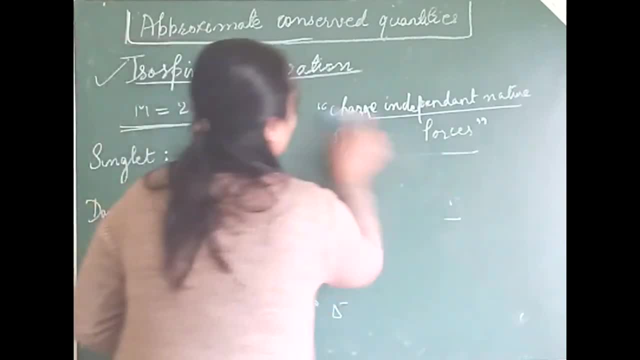 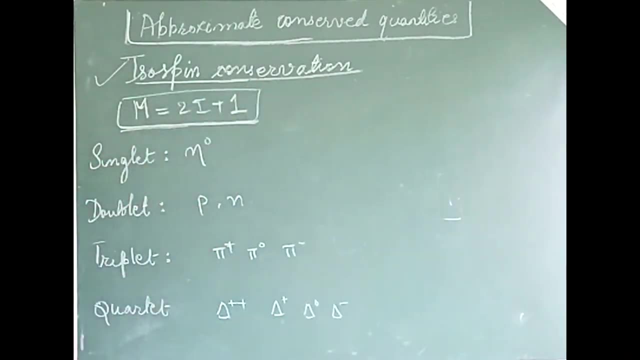 arises because of the charge independent nature of your nuclear forces. okay, So now, when we are dealing with isospin, this formula becomes important. where you have m equals to two I plus one, So this formula will help us to identify the isospin of your different. quantities right, So now we have different multiplicities, right. First we have multiplicity, right, So now what is the multiplicity of electric current? So this is about the energy current. So it is about energy current right. So we have energy current, right We have. 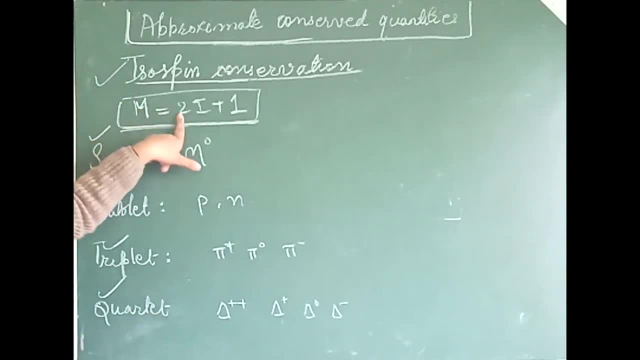 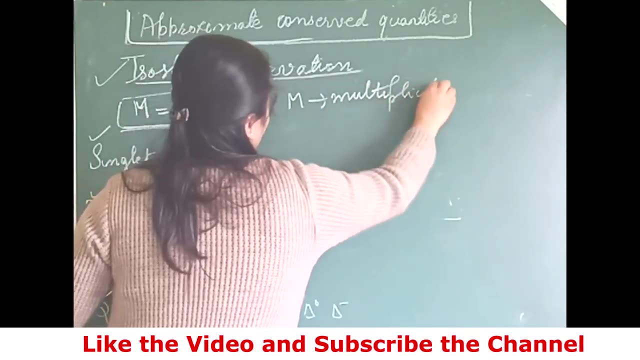 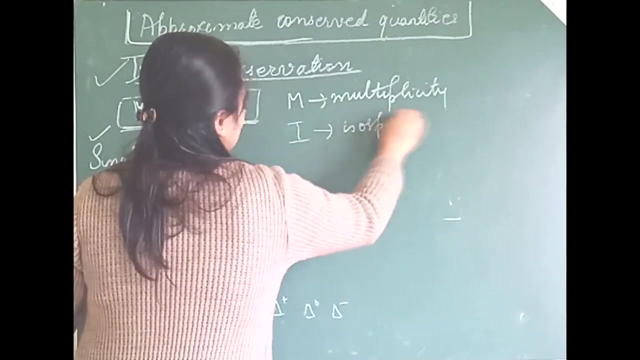 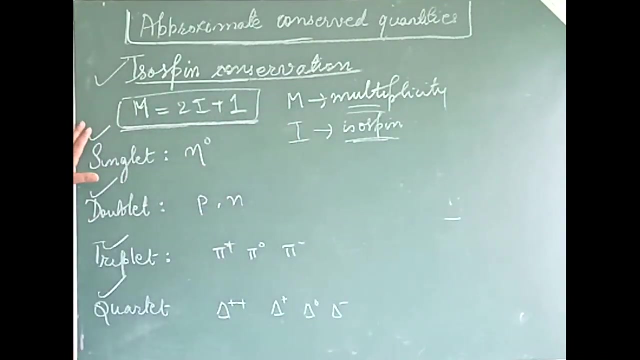 Okay, First let me explain what this formula means: M equals to 2I plus 1.. Here your M is multiplicity- And explain what is multiplicity- And your I is isosceles, Right? Okay, Now we have singlets, we have doublets, we have triplets and then we have our quartets. Now, what are singlets? Singlets meaning this particular family is going to have just one member in its family, Right? 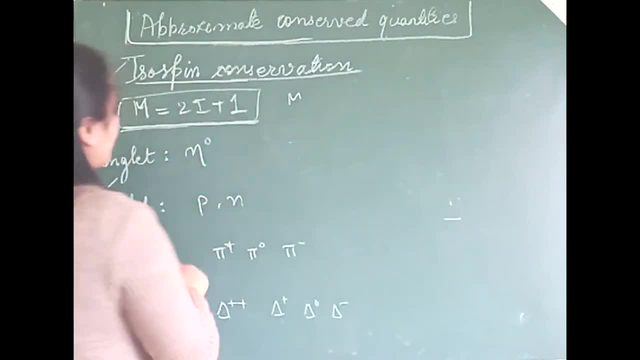 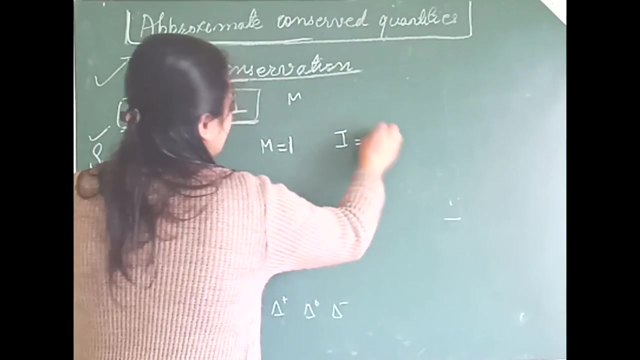 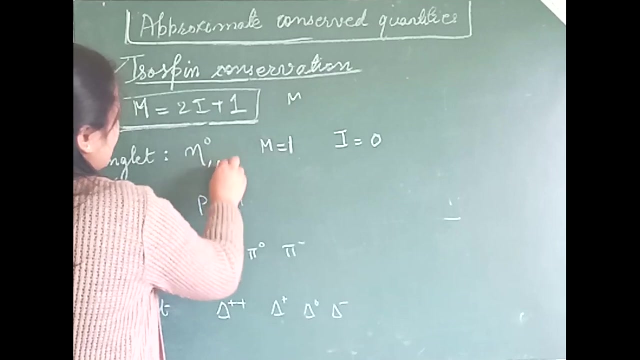 So by making use of this formula here, my multiplicity is 1, because I just have one member in the family. For this, if I calculate using this formula, I am going to get my I to be 0.. So the isosceles spin of this particle, eta 0, is 0.. So another such particle is going to be your lambda 0 or your omega minus 1.. Right, 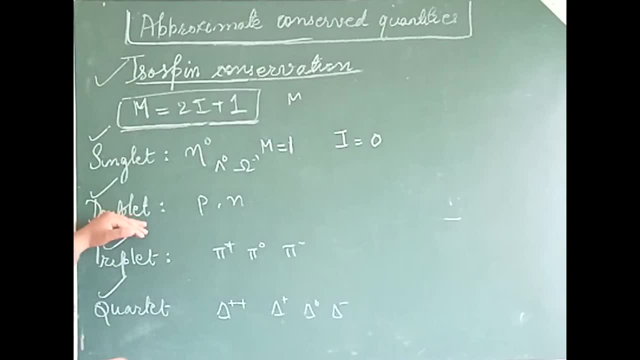 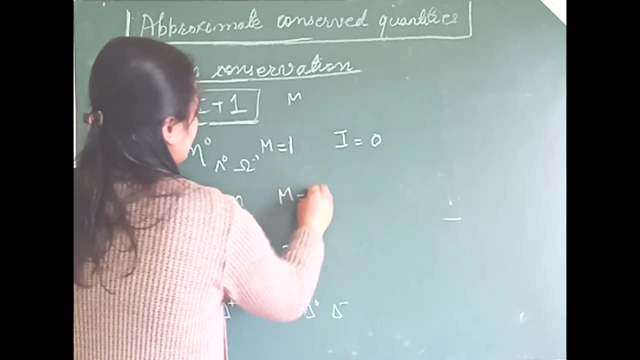 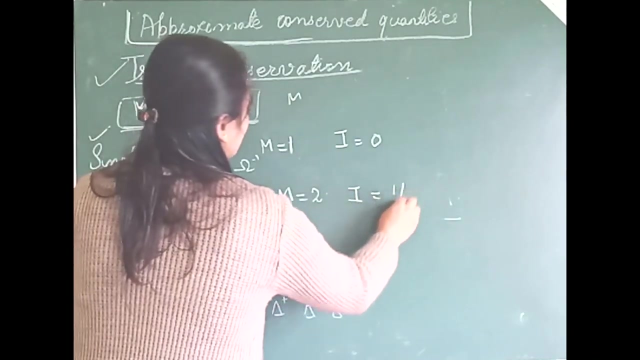 Okay, Now let us calculate doublets. Doublets meaning this particular family is going to have two members Right, For example, your protons and neutrons. So where your multiplicity is going to be 2 and your isospin, using this formula, is going to be dalla rite, So it is 2 minus 1. divide by 2 means it is half. 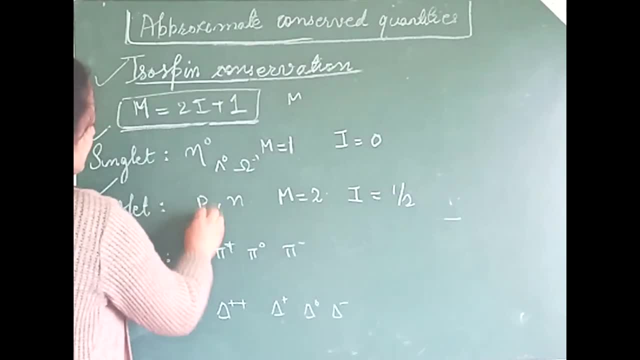 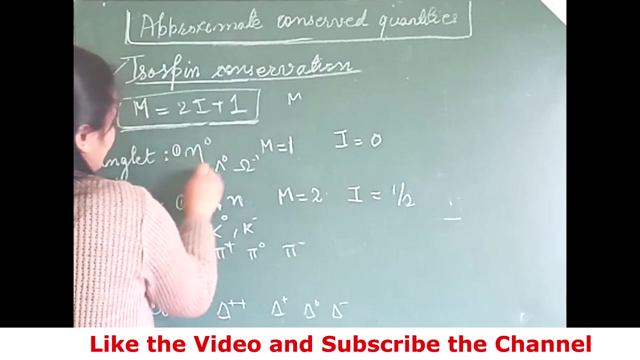 Okay Now. another such example for this protons and neutrons doublet will be use is k0 and k minus Right? Okay, This is example 1 and example 2.. For singlets, this is 1,, 2 and. 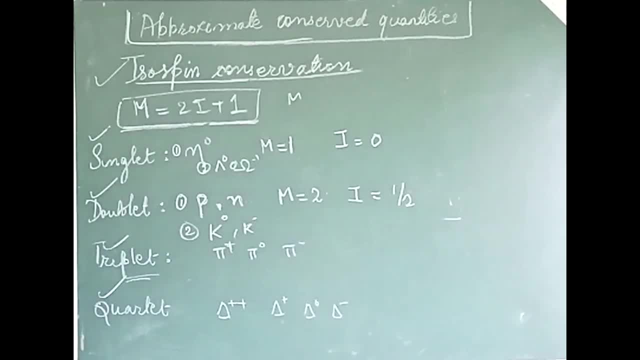 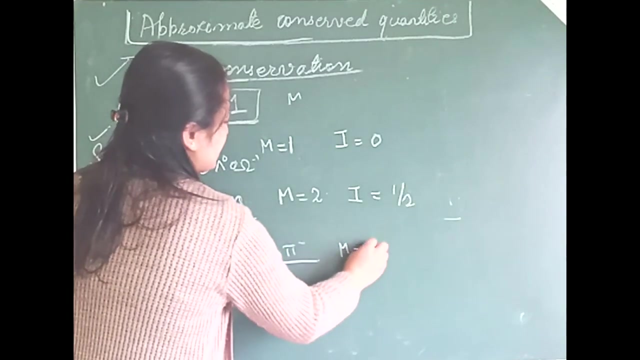 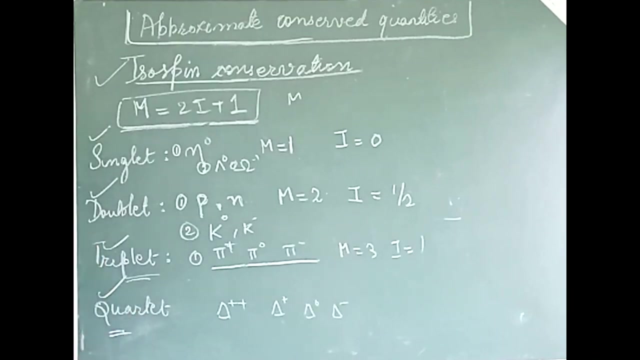 25. example Now coming to triplets. So triplets meaning there are three members in the family right: pi plus, pi zero and pi minus. So my own family is going to have three members: pi plus, pi zero, pi minus. So my multiplicity is three and hence my i is one. right Now I have my 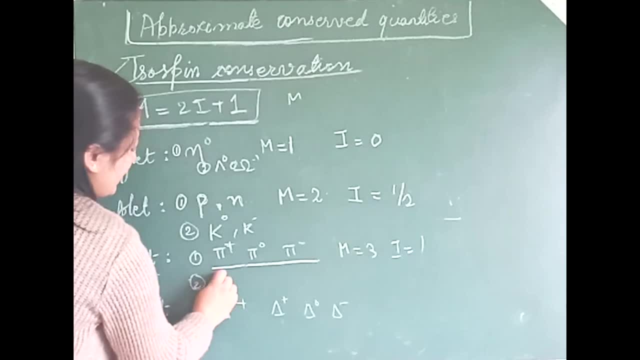 quartets. So here the other example could be your sigma plus, sigma zeros and sigma minus, So quartets. So when we are talking about quartets, so this is one such example- the family is the delta family, where there are four members in the family and your multiplicity, hence 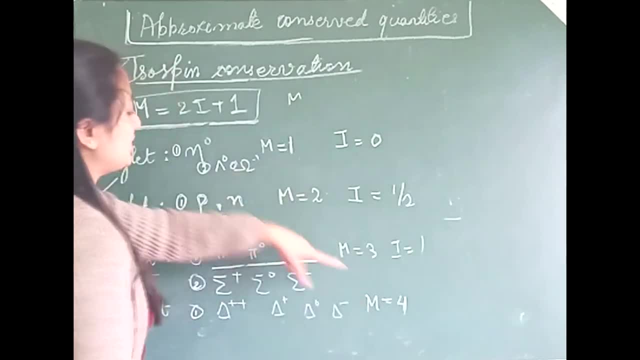 is four. So if I am going to make use of the value four over here, I am going to get my isospinas Three by two, right? So all the members in my sigma family is going to have my isospin as zero. The members in doublet family is going to have my isospin half Triplets are 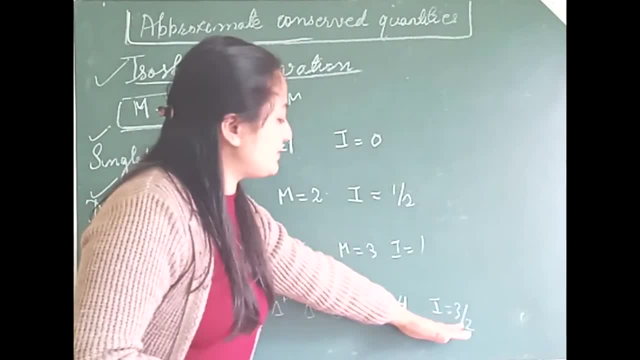 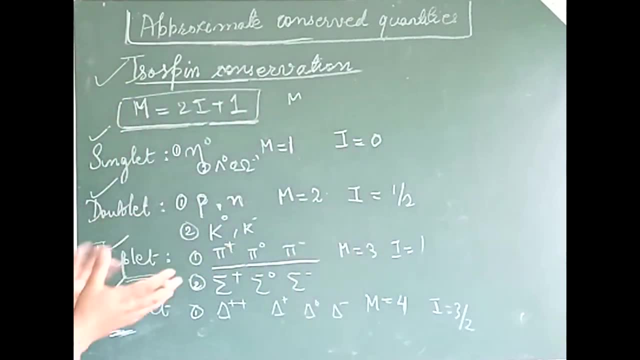 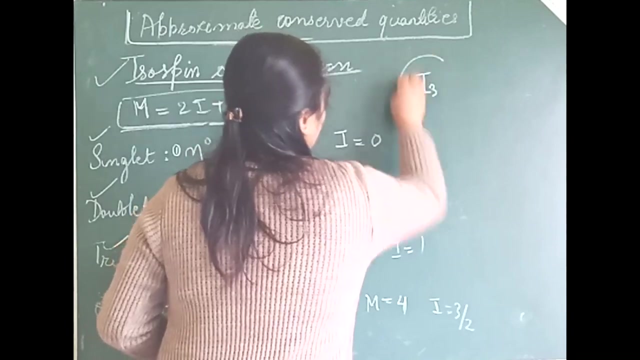 going to have isospin one, and quartets are going to have isospin three by two. Okay, Now, still, I am not able to distinguish whether it is proton or neutron, because the isospin is running in half, right. Okay, So I introduce another quantity, which is called: 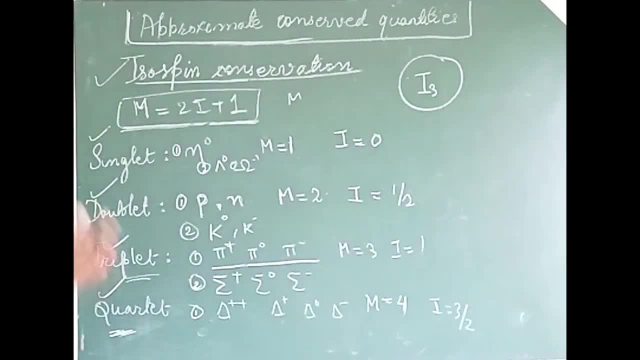 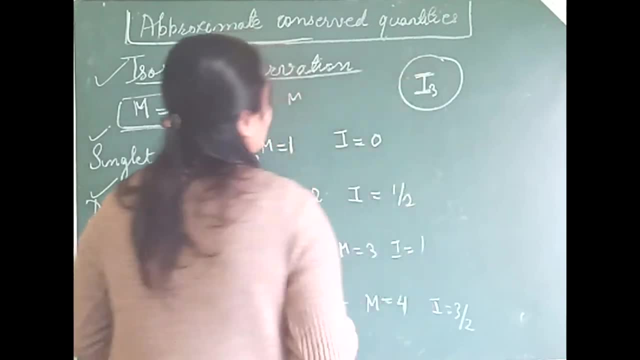 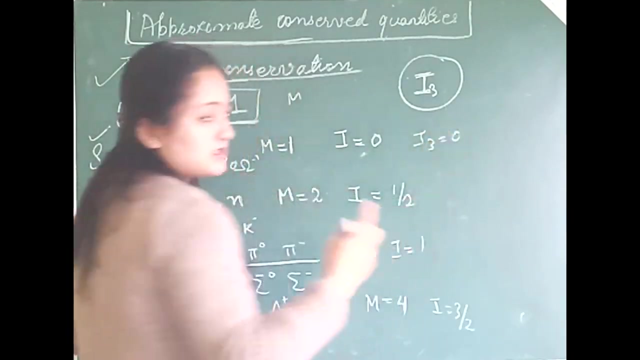 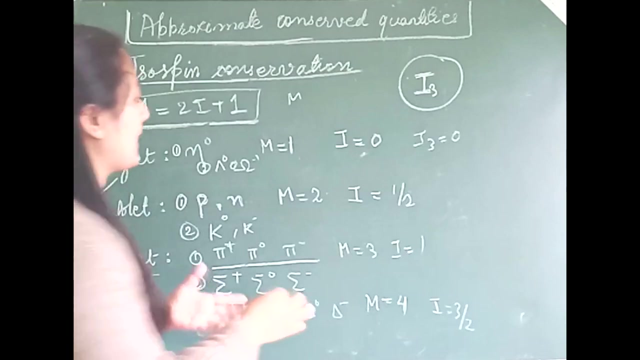 I three, which is the component of isospin in a particular direction, right. So let me see how to assign this I three values here. So here I three is zero because just one particle right. And here so my isospin I three is going to vary from, is going to vary in steps of. 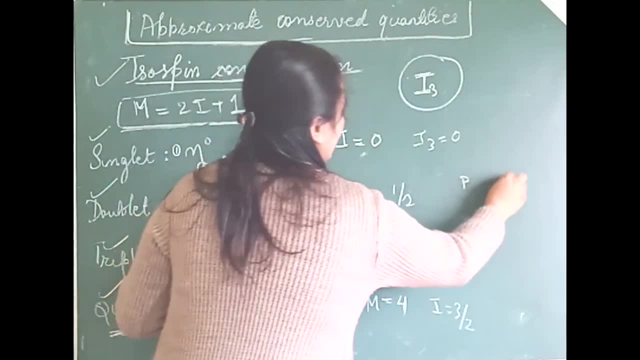 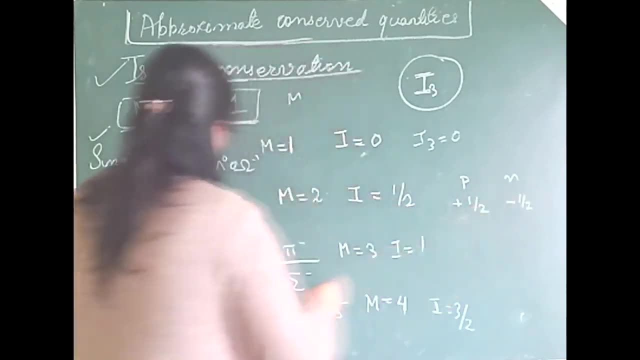 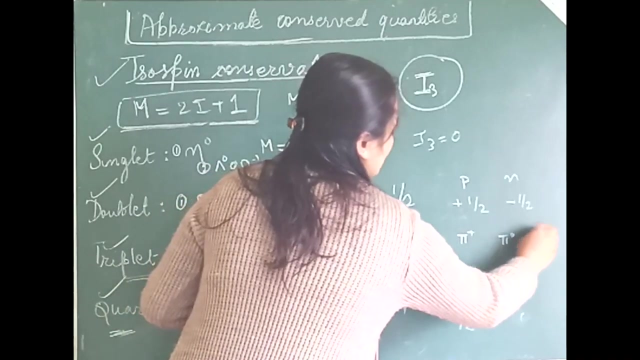 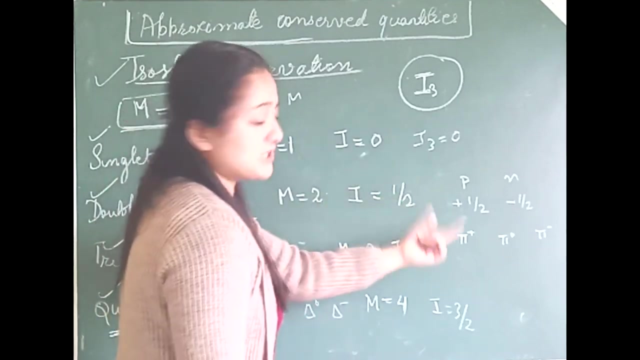 one Hence here. proton And neutron will have my isospin as plus half and minus half, And when we are talking about the triplets, the members of the this triplets, So see. for example, I take pions, So my pions. here is one right, So I give the highest number to the positively charged. 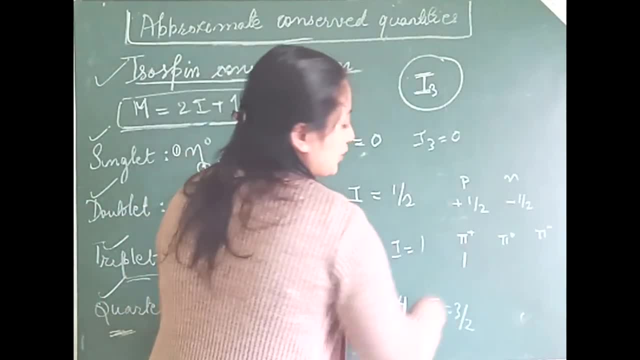 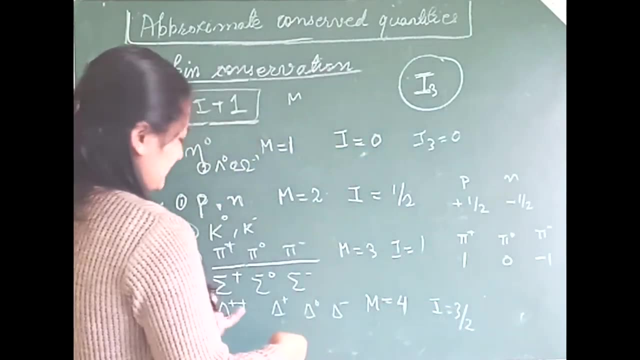 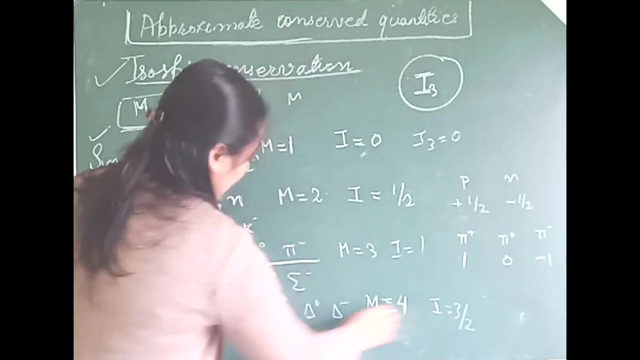 particle, Particle with the highest charge. So meaning I am going to give one here, zero here and minus one. They are going to vary in steps. So one and I have my deltas where. okay, let me write it over here. So your I is three. 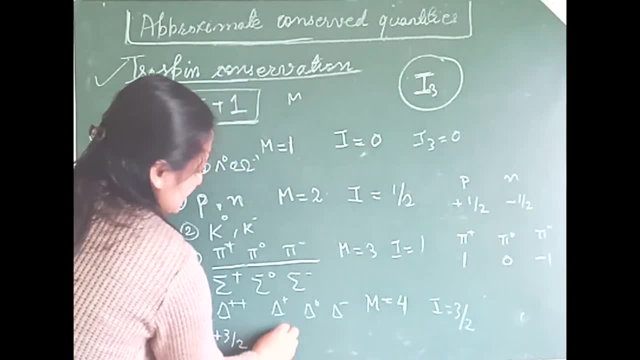 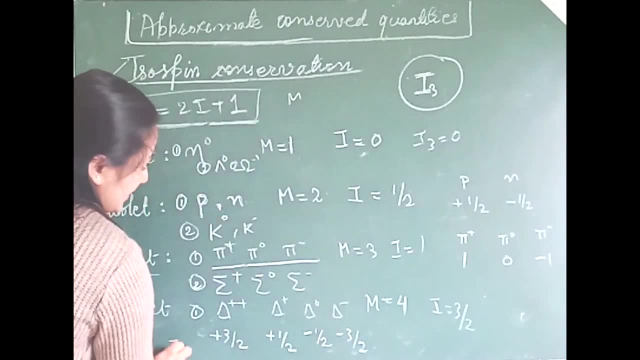 by two, So it's going to be plus three by two plus half, right minus half and minus three by two. So these are the I three values. Okay, So these are the I three values Here. these are the I three values And again, these are the I three values for the. 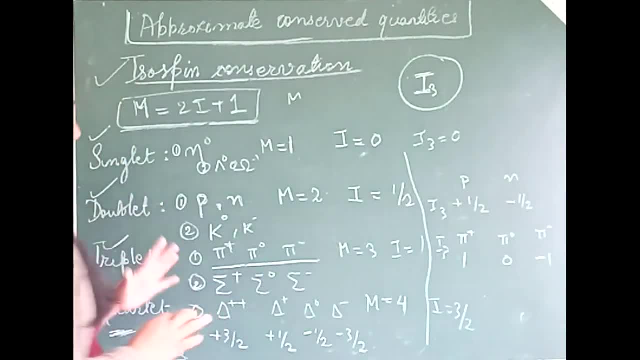 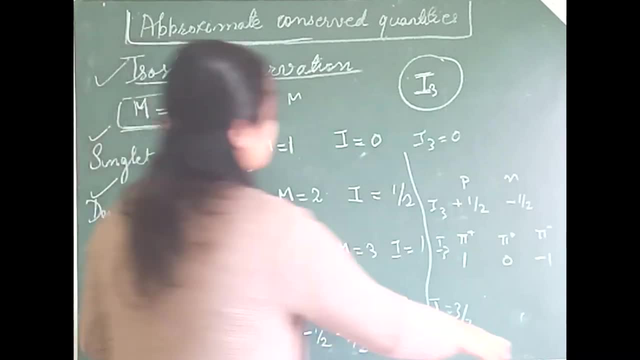 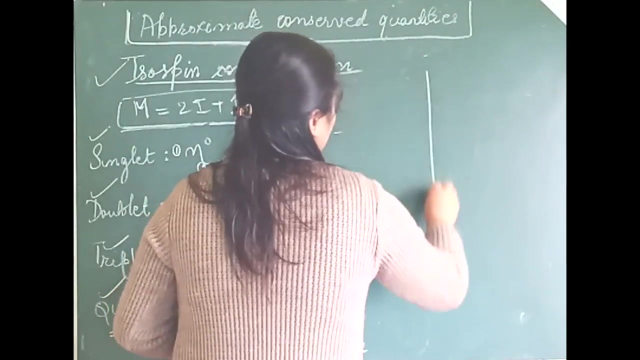 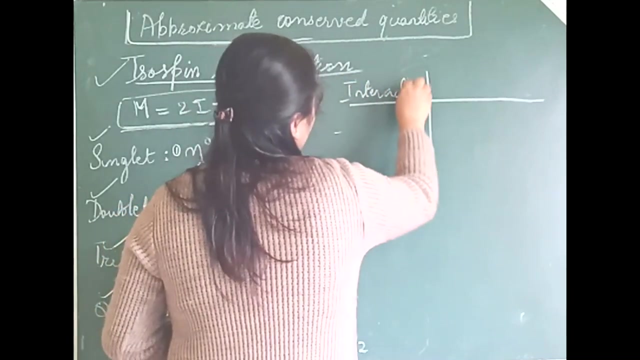 Now, So see these. like the name suggests, these are all approximate conserved quantities. So these are the quantities which may or may not be conserved in all possible interactions. So So let me talk about interactions here. Right, I will give you the table and the conserved. 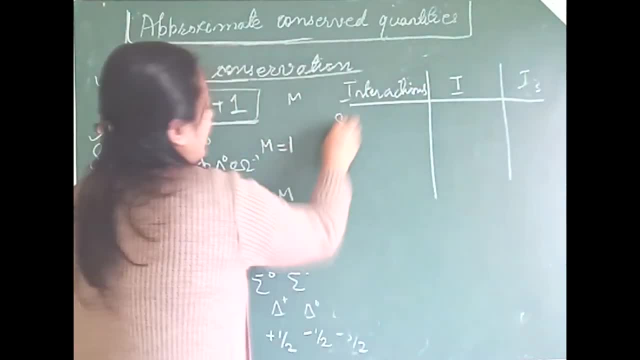 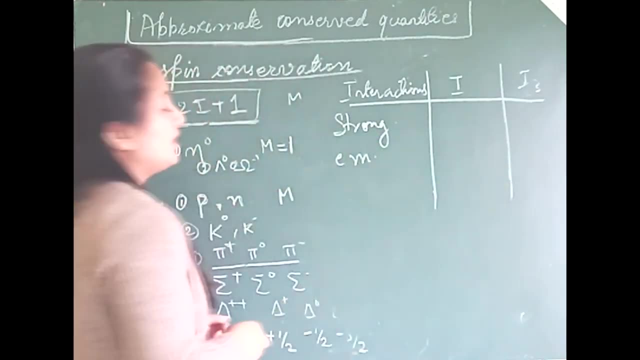 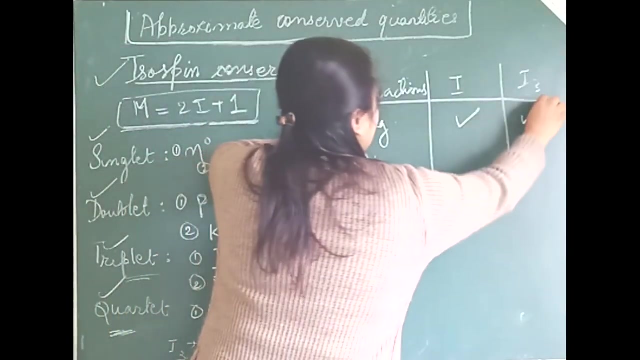 quantity, I and I Right. So I have my strong interaction, I have my electromagnetic interaction, EMD, noting the electromagnetic interaction, And then you have your weak interactions. Okay, So strong interactions, I and I, three, both are conserved. Take meaning they are conserved. 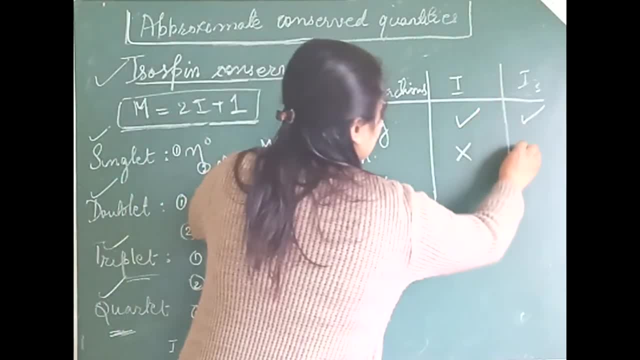 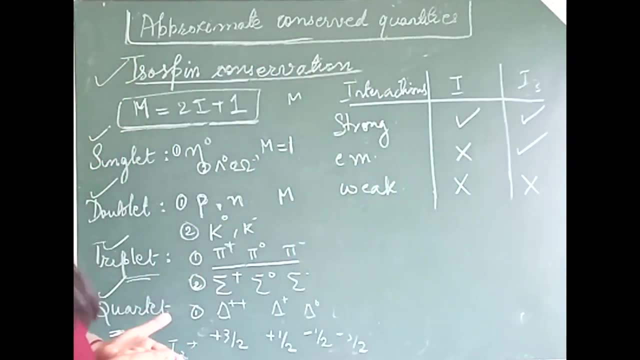 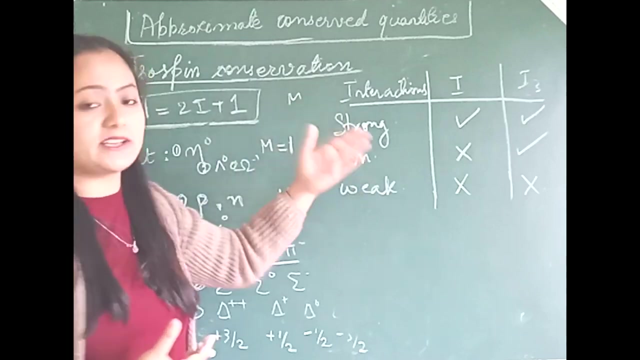 In electromagnetic interactions my I is not conserved, but my I three is conserved. In my weak interactions both of them are not conserved. So So I can identify I three values whether they are conserved or not. by checking that I can identify whether I am talking about a strong interaction, an electromagnetic interaction. 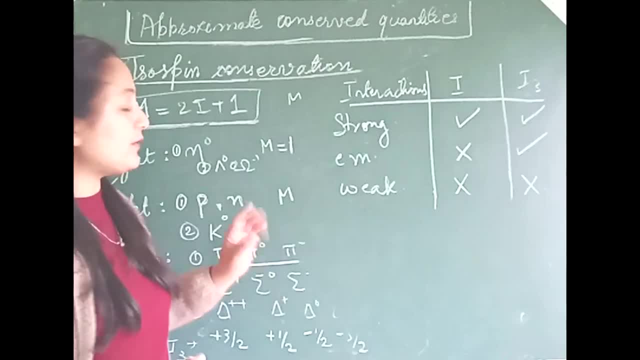 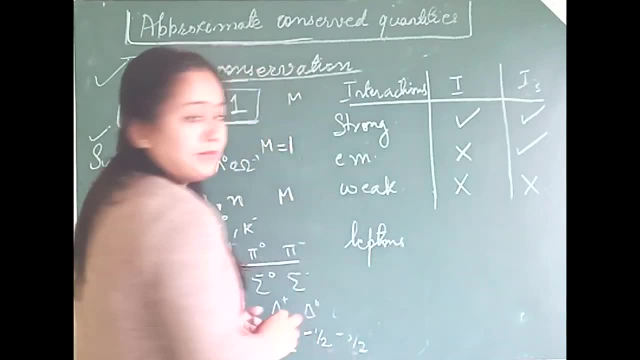 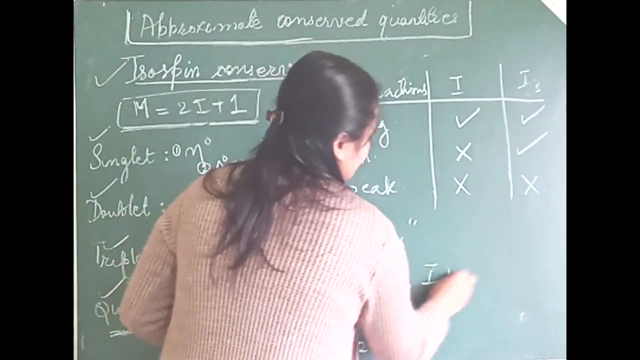 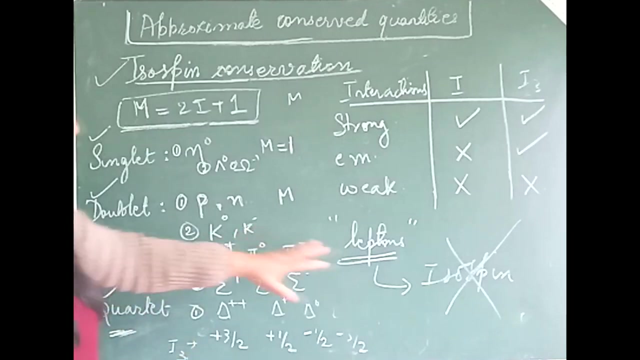 or weak interaction. So this is it. And one important thing to remember is Your left turns, Right, They do not have isospin. So when it comes to left turns, they do not have isospin. Why? Why left turns don't have isospin? Because isospin, like I said in the I said earlier, these isospins, 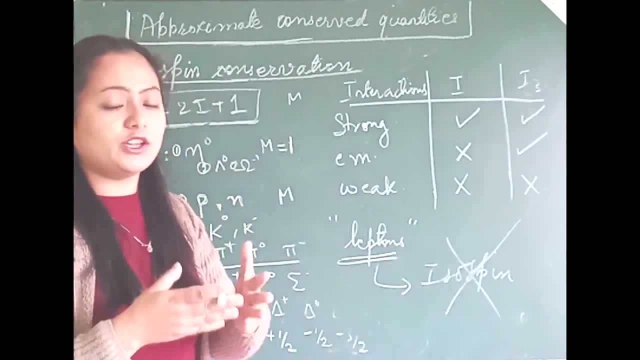 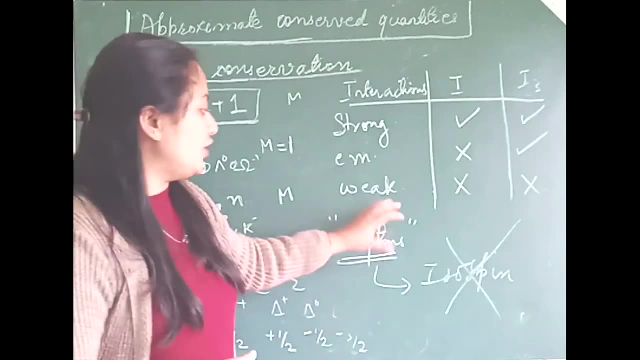 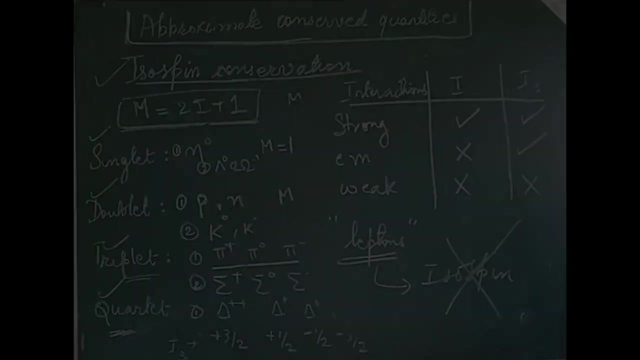 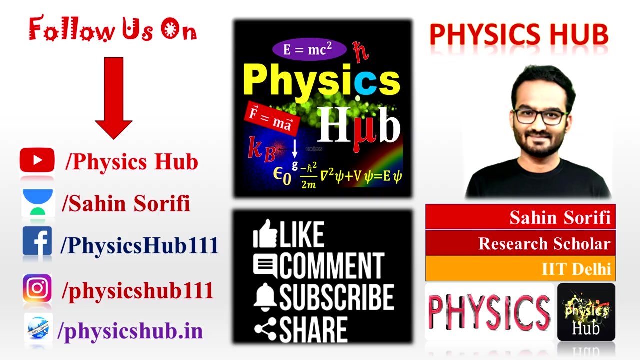 are. they originate because of the charge independent nature of nuclear forces and left turns. they do not take part in your strong interactions, Hence your left turns. they do not have your isospin Right. Okay, Let's leave the gaanza and get back to your right turns. Turns existẹ. 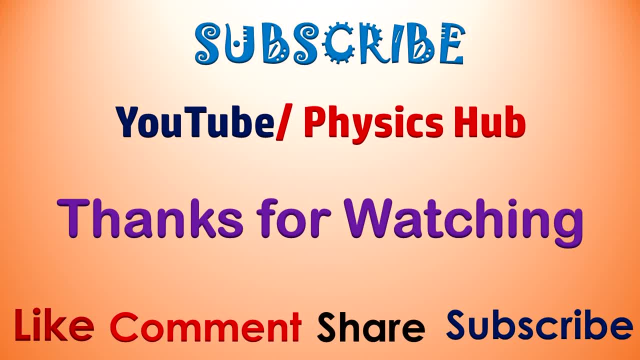 over there. Do you see the left turn stress? True? So let's do it again. So open the left turn stress. Thanks for watching. 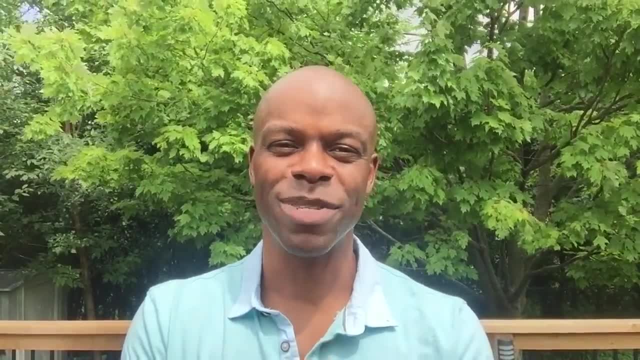 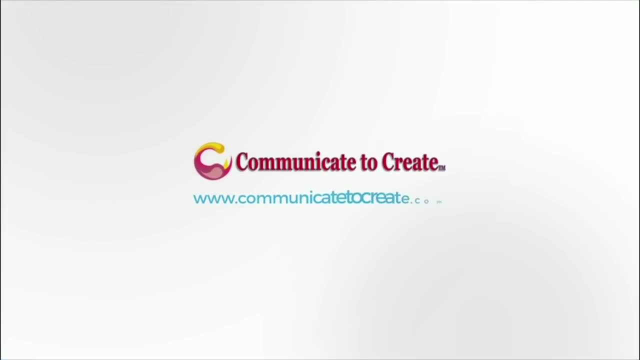 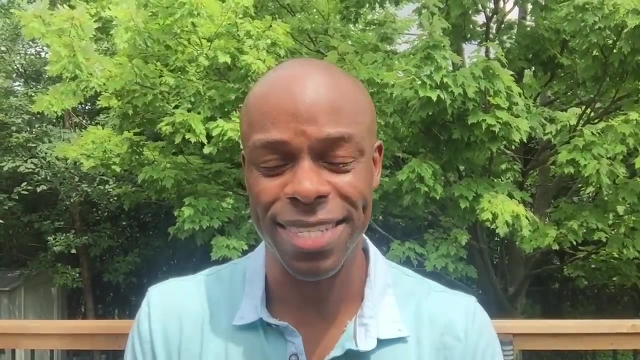 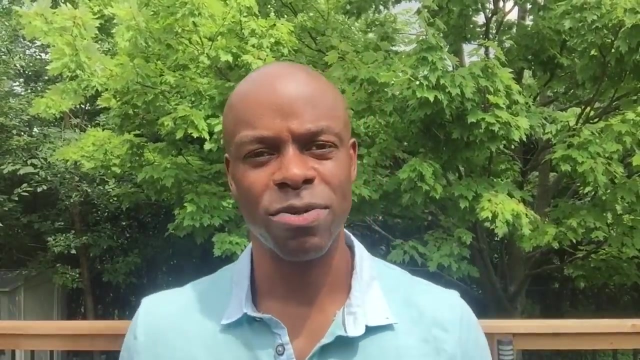 In today's video: five public speaking tips for kids. Public speaking tips for kids, for youth, for students, for debates. I see the same mistakes over and over again And as I coach students, whether it's in Toastmasters or outside, on how to deliver speeches, I've done it for a while now, for a few years now, And I see. 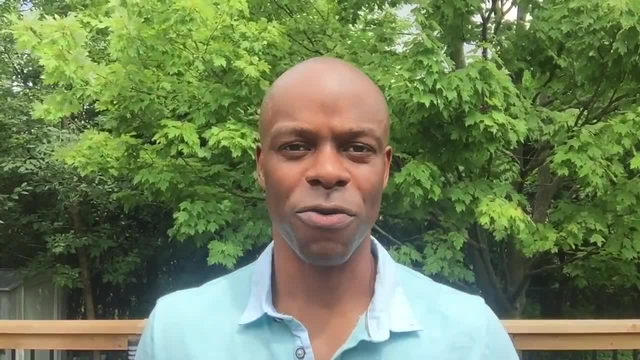 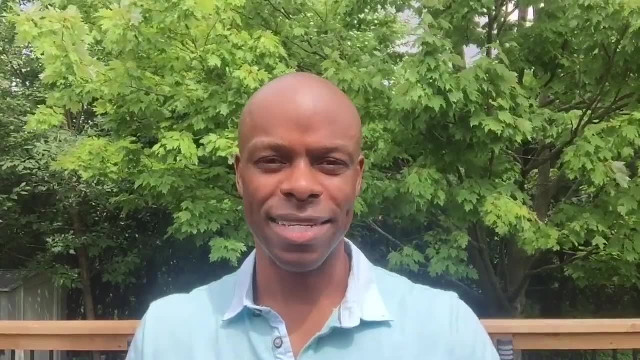 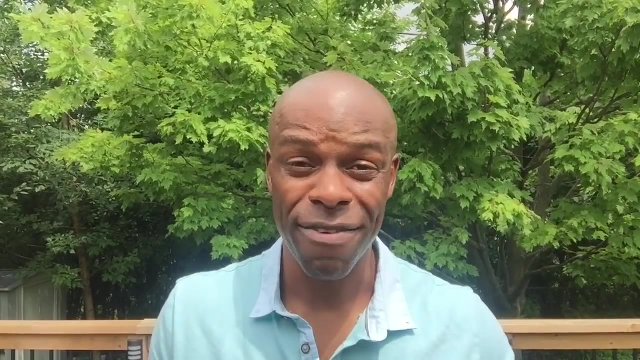 the following five mistakes, made over and over again, And I believe it's what separates the speakers that end up winning competitions or even just presenting with confidence, from those who get up present, sit down and say: I never want to do this again. If that is you, you'll be a lot less.